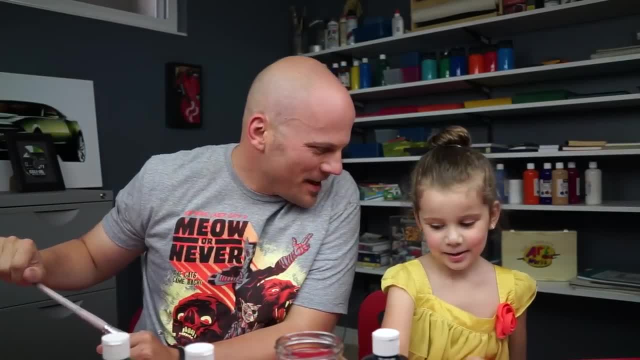 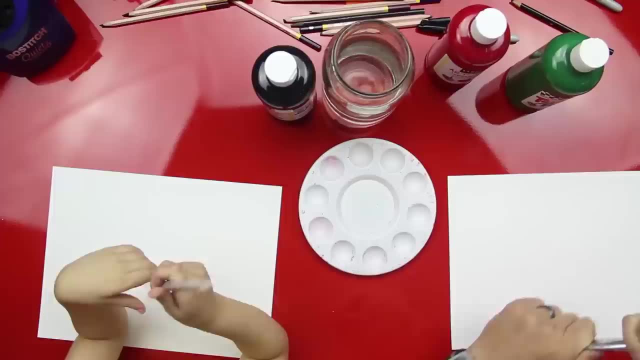 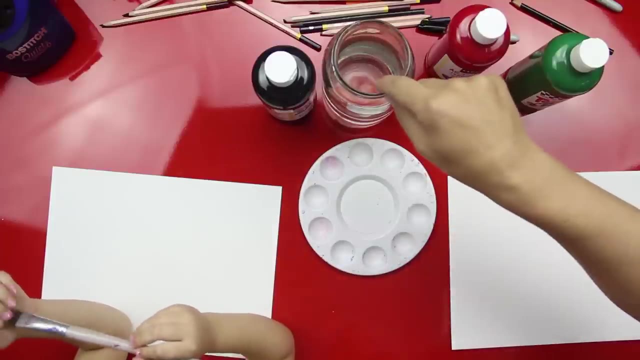 All right, so watermelon's your favorite thing to eat? Yeah, In the summertime, Yeah, Yes, it's my favorite thing too. You ready to paint? Yeah, All right. what do we got here? What colors? Black, Black, Red, Red, Green, Green, Yes, And we got. what's this? 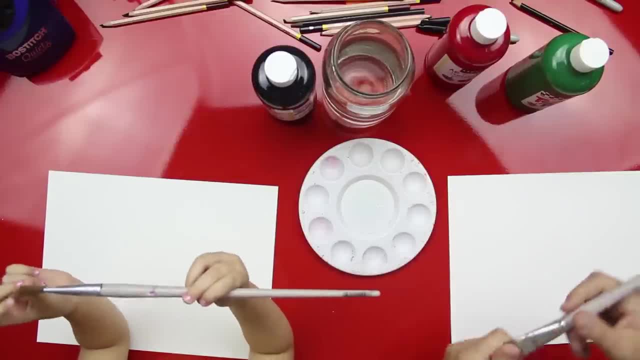 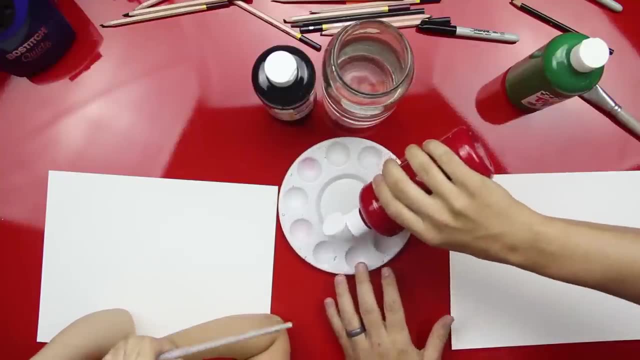 Some water And this is a paint tray, huh Yeah. Okay, you ready, Let's get some. we're gonna start with red. Does that sound fun? Yeah, And we're gonna draw. this is gonna be really cool, We're. 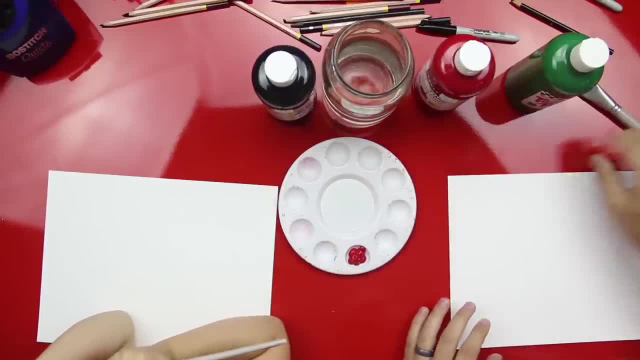 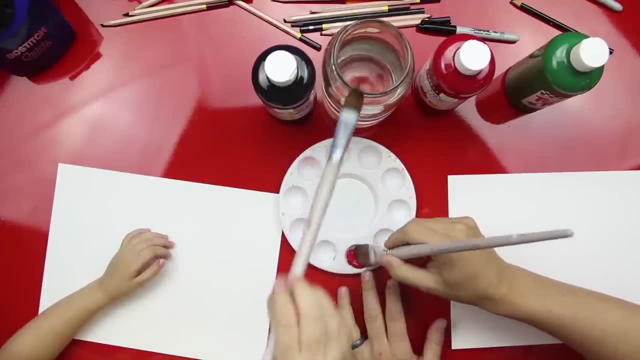 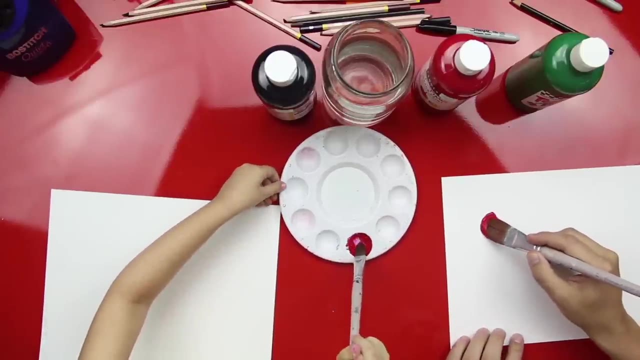 gonna do this a really simple way for young art kids like yourself, Hadz, That'd be fun. Here we go And get a little red on your paintbrush And watch me Watch the first step. We're gonna do a big giant U. Can you do a big giant U? 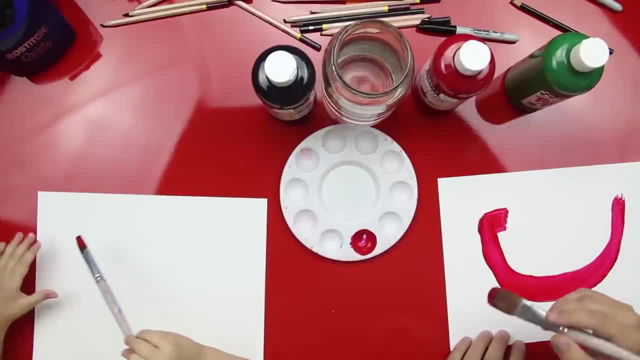 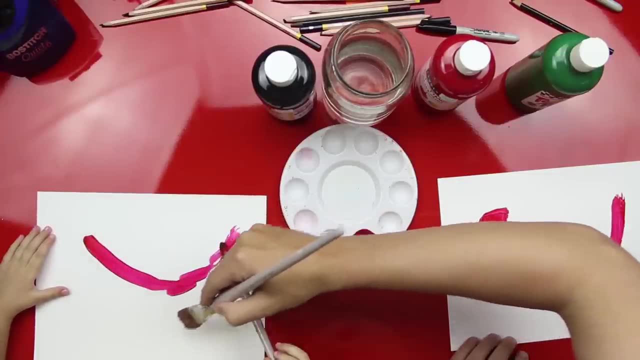 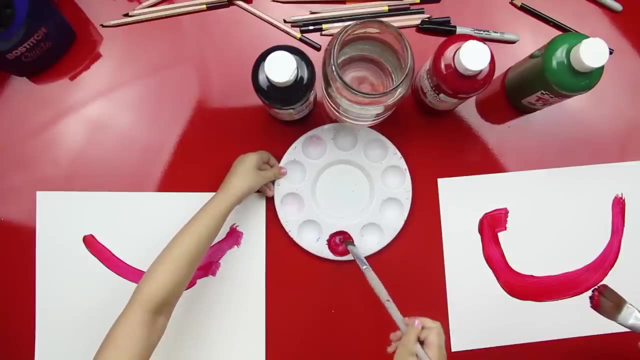 Oops, I almost did the next step. Do a big giant U. Yes, You can go even further down. Go all the way down here. You wanna get a little more paint? Get a little more paint on there? Yeah, Good, So come all the way down here and then back up like a big smile. 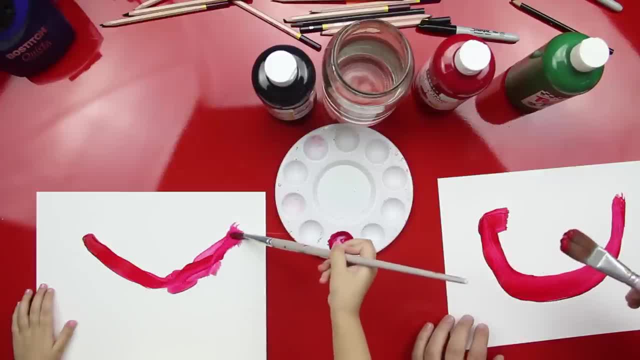 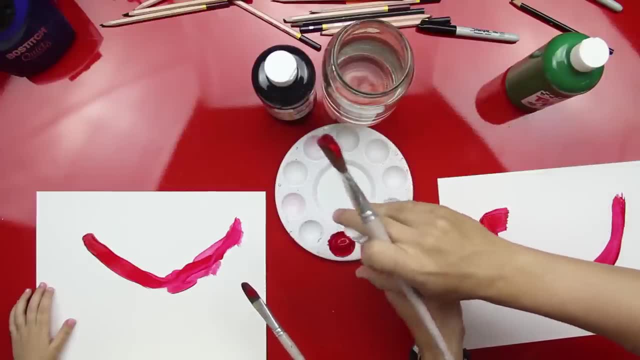 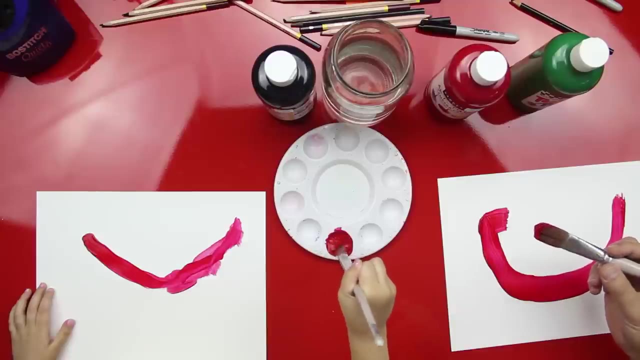 There you go. Good job, Hadz. All right, okay, you ready for the next step? Yeah, We need a little more red. Let's get some more on there, And we're just using tempera paints for the, for the parents and the art kids at home. We we like using tempera. It's a good paint for kids. 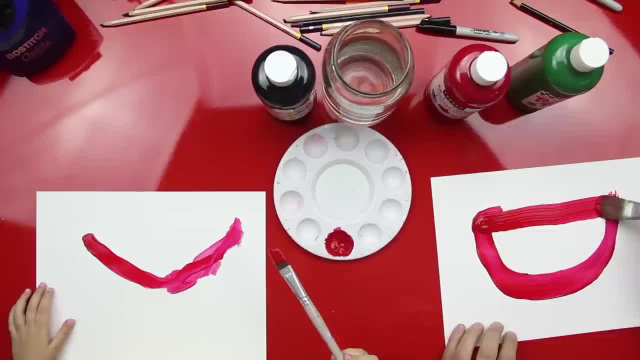 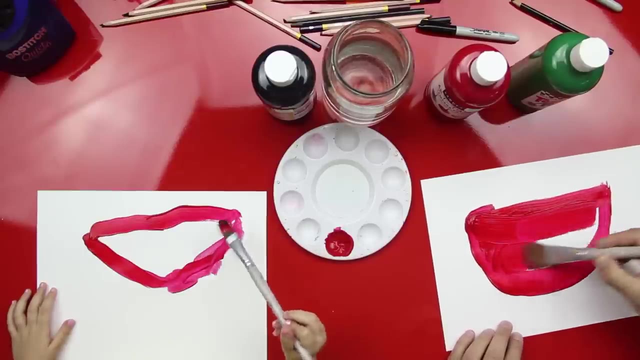 Ready for the next one? Yeah, Okay, next step: we're gonna go straight across on the top. Connect the top. Good job, Good. You even flipped over your paintbrush to get more paint. Okay, next step. Color it in. Color the whole watermelon in. Look how bright. 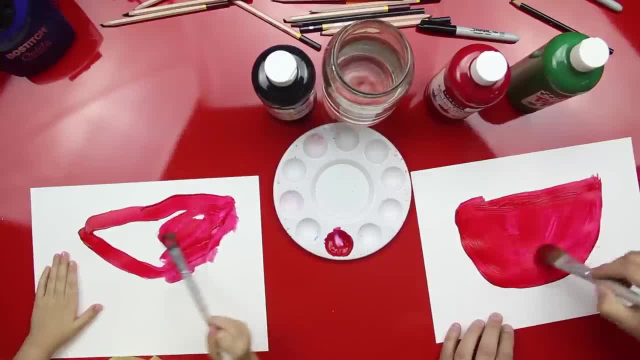 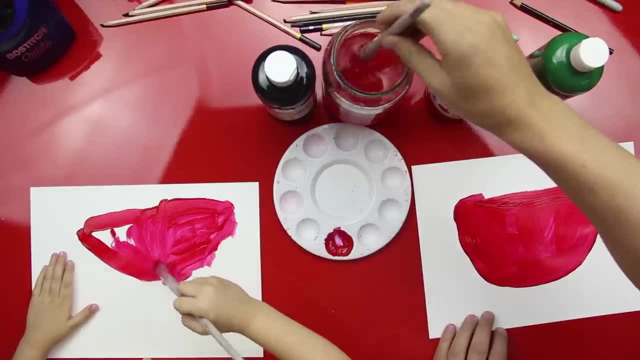 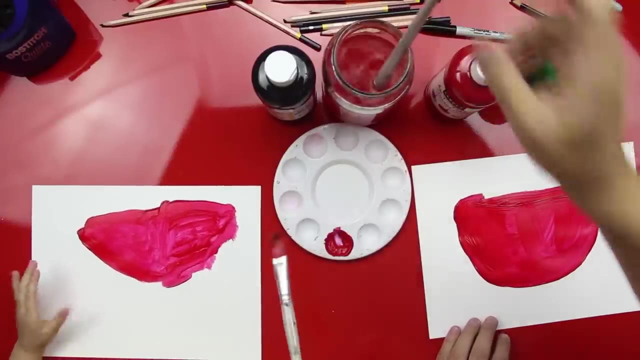 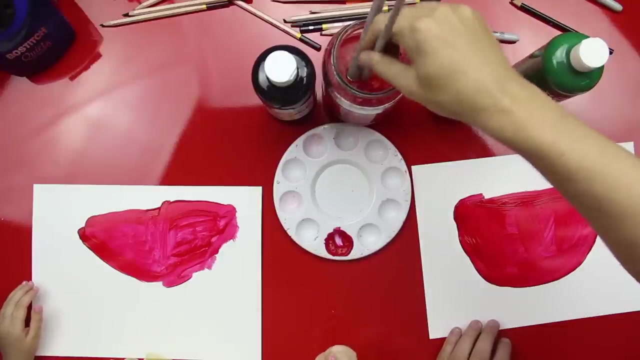 that red is. That's crazy, huh. Well, you're doing a good job. Does it look like a watermelon yet? No, Almost Okay. put your paintbrush in there and then we'll get all the paint off. I'll help you so we can do it a little fast, faster. There's a video. 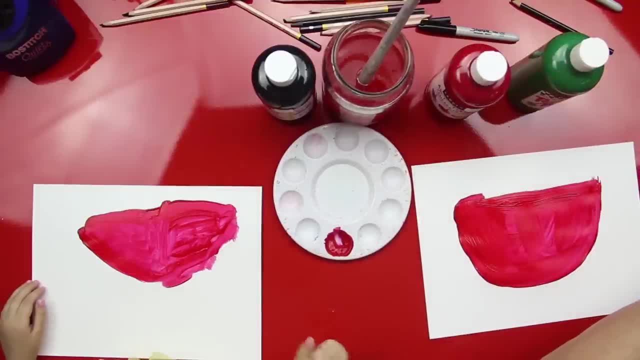 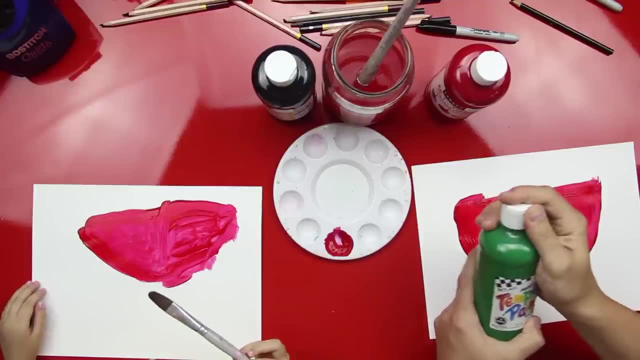 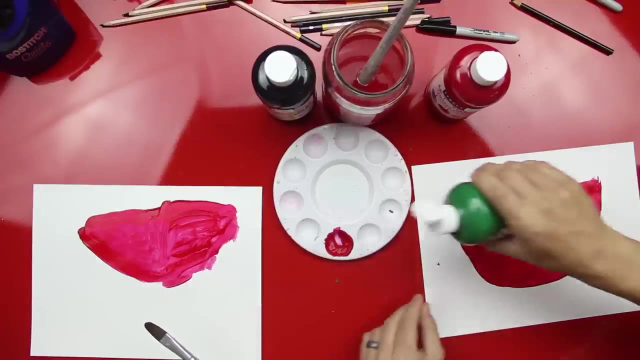 There we go. All right, okay, now you ready for the next color? Yeah, What's the next color? on the watermelon, we're gonna do Green. Yes, green. How'd you know, Are you good? Oh, got a little dry paint here. We'll move that off to the side. Okay, all right, we're gonna put. 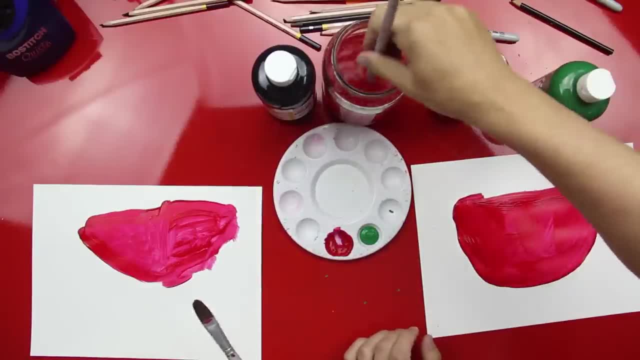 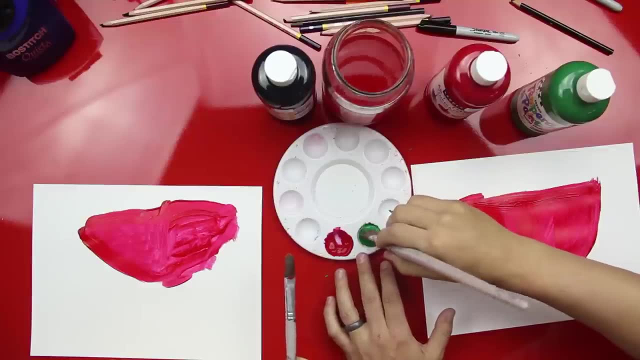 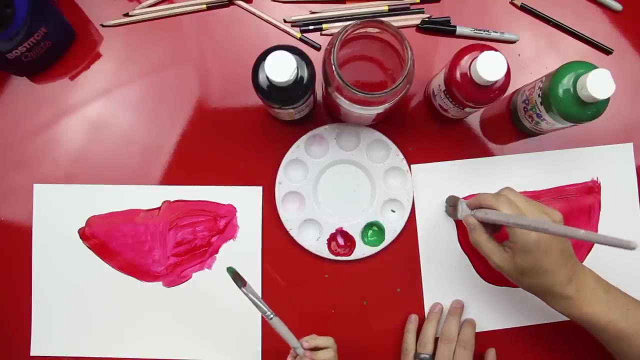 a little, a little green in there. Get my paintbrush and then watch this. We have a little green on our paintbrush. Go ahead and get some on yours. Good job. Okay, we're gonna start over here and we're gonna go right on the outside. 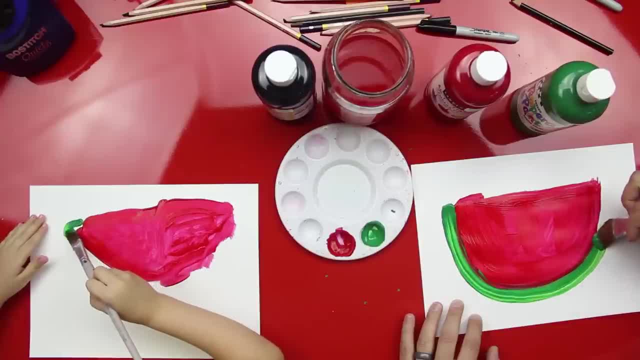 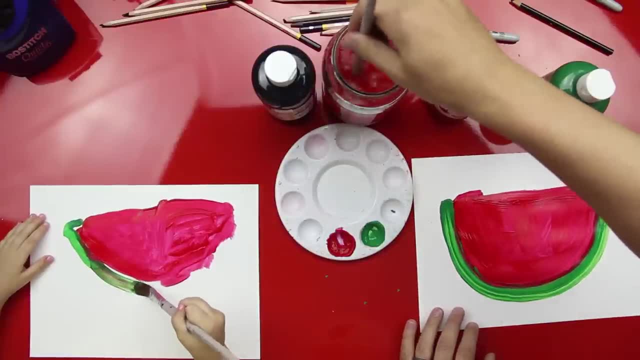 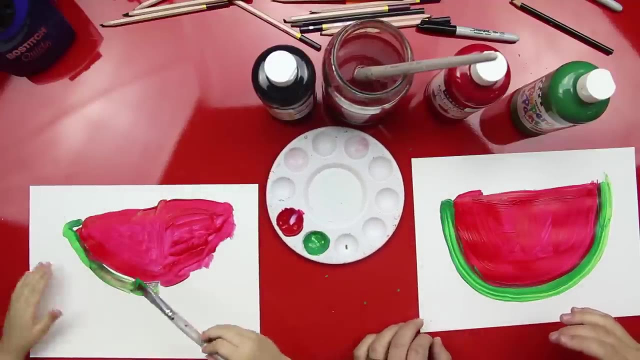 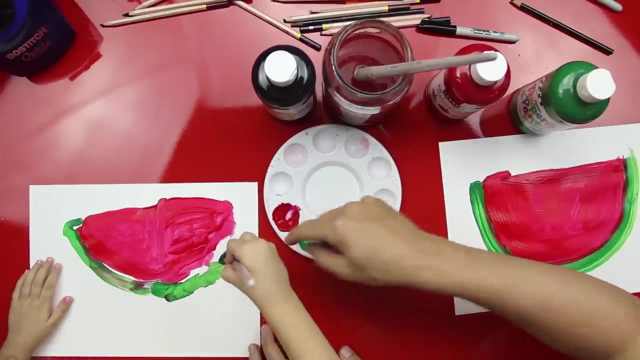 of the red and trace the outside of the watermelon. Good job, Keep going. Get a little more green. You're kind of running out Now. does it look like a watermelon? Yeah, A little bit. Yep, Good job, Keep going. Just go all the way up. 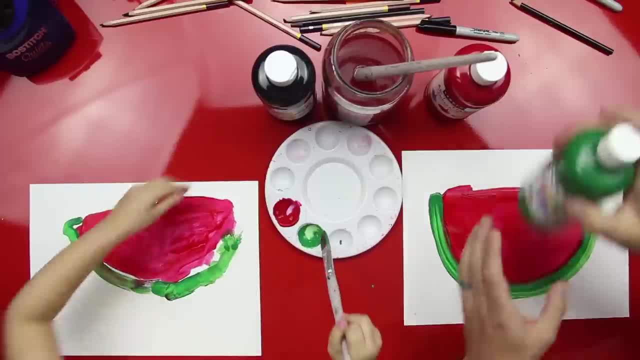 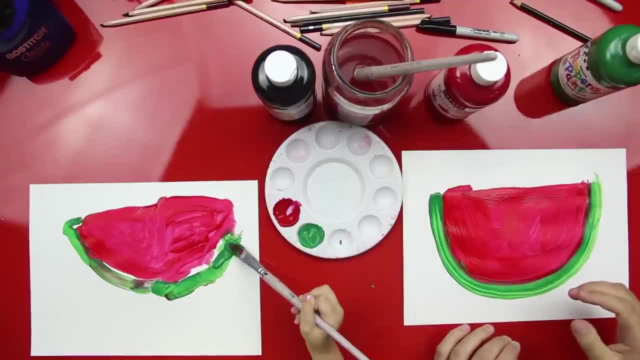 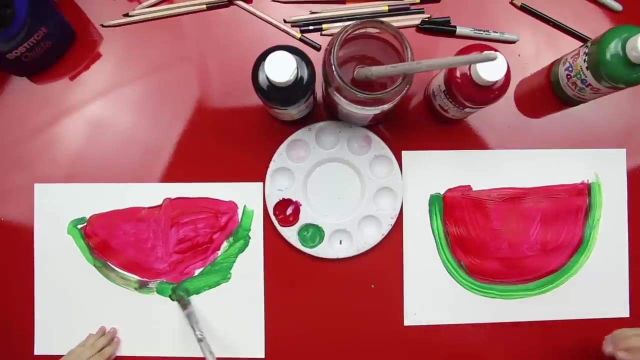 Yes, go all the way up here. A little more green Here. I'll even get some more on there. There you go. I probably gave you too much. That's okay, We can do it again. Do another watermelon after the video, That'd be fun. Okay, good job, Hads, You did awesome. 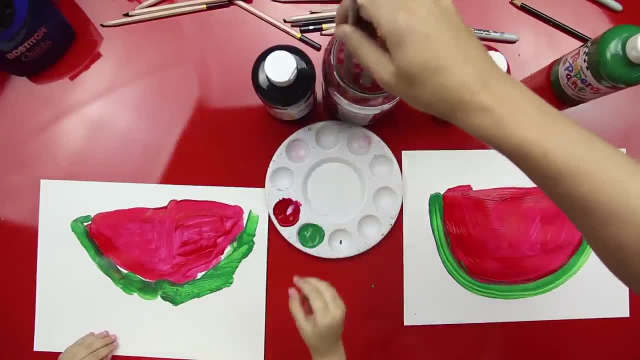 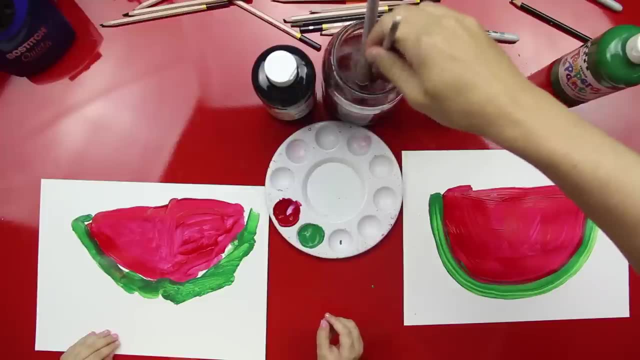 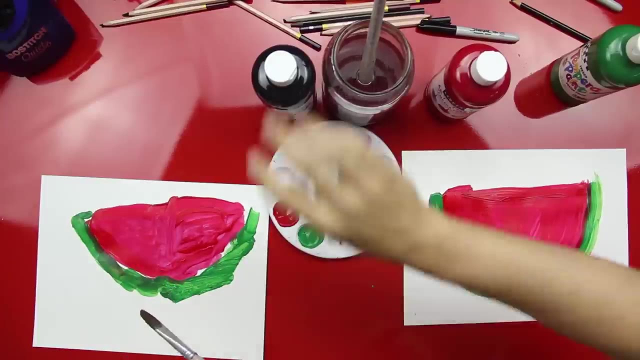 Good, Okay, put it in here and I'll help you rinse it out. Oh, we got watermelon water. Alright, what's our next and last color? Here's your paintbrush. Black, Yes, black. What are we going to do? black for The seeds. The seeds, yes, Okay. 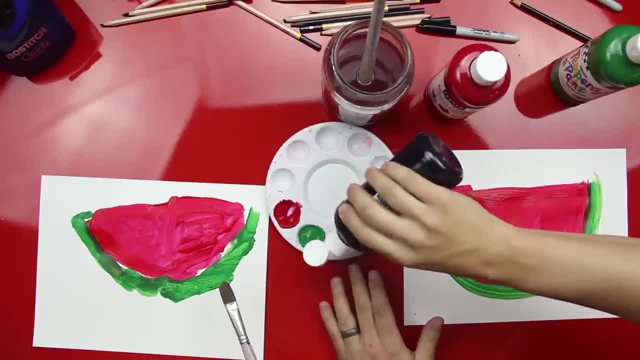 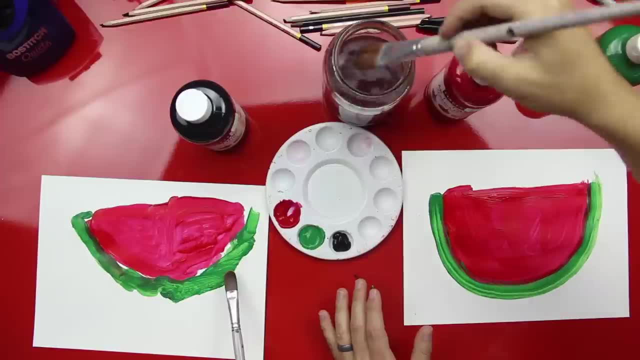 Our kids at home. you guys could use a smaller paintbrush if you want. We're just going to use these because you can. I'll show you a little trick. If you don't have a different size paintbrush, You've just got a big one.